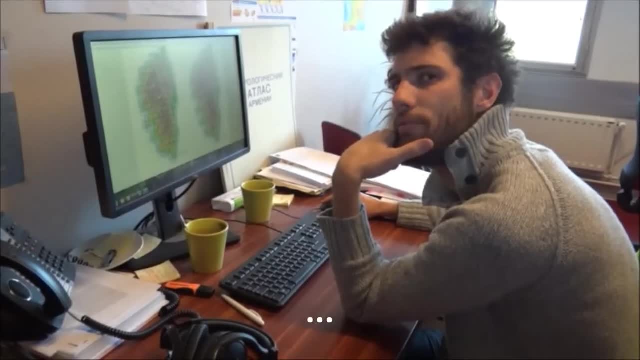 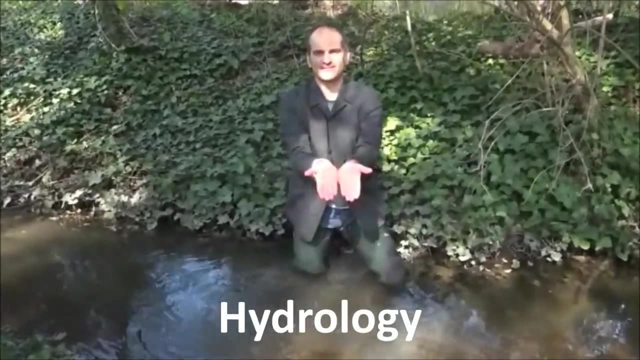 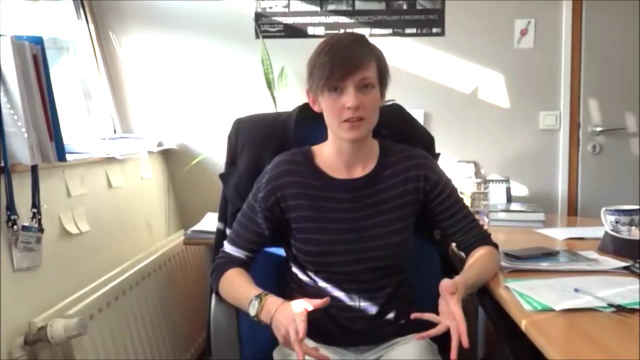 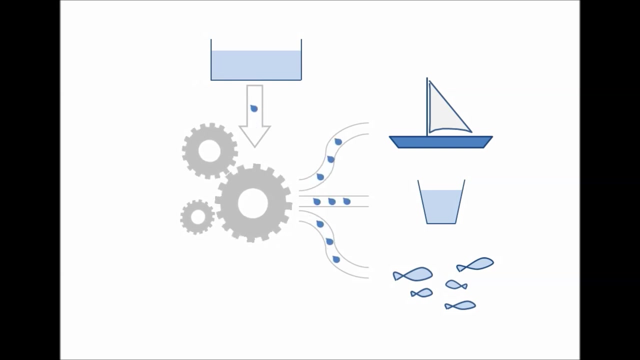 Dams. You work here. Go back to work now Hydrology. Well, I sure work in hydrology to forecast low flows and droughts and propose tools to decision makers to manage their reservoirs. Suppose we have a surfaced water reservoir that provides three uses with water. 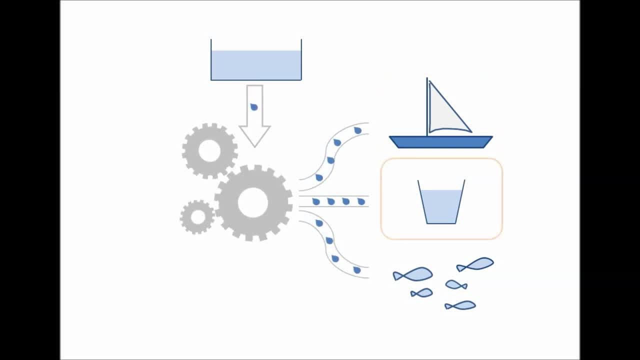 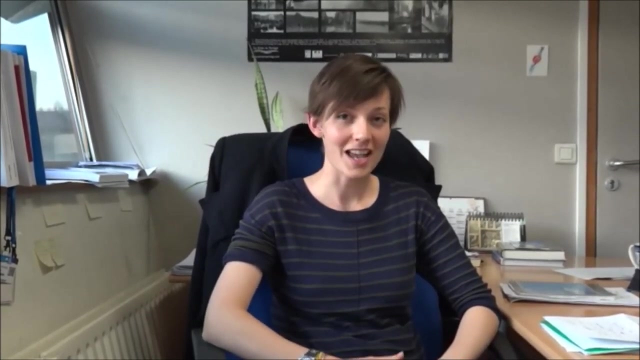 Navigation, Drinking water And fish migration. In summer, the volume of the reservoir tends to decrease unless water is available for allocation. In the case of a drought, we can even reach situations when water scarcity prevents the different uses. My PhD focuses on the reservoir of the Arcel Dam in Brittany, France, which I had the chance to visit. 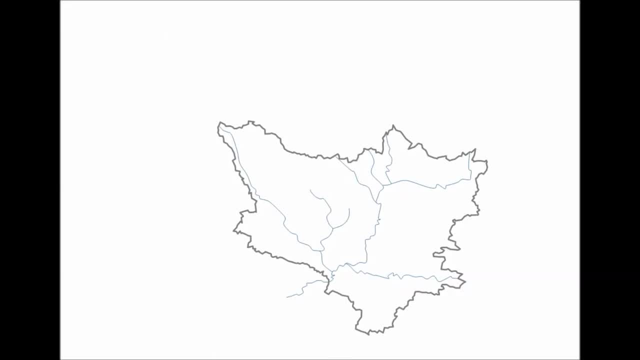 But mostly I get to do this. This is the hydrological catchment. This is the hydrological catchment upstream, our reservoir. In winter, precipitations are usually more intense, Rivers fill up and so does the reservoir. In summer, precipitations tend to decrease. 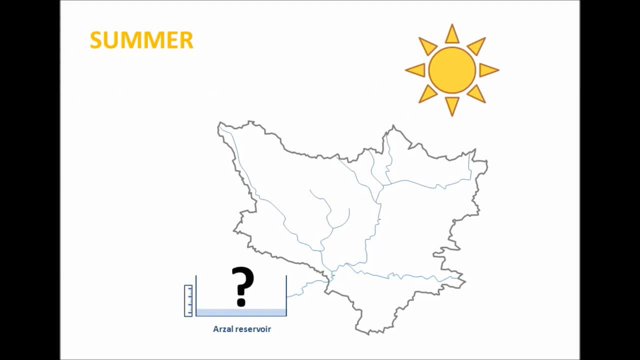 We want to quantify the allocatable water volume in the reservoir for the coming weeks. To do so, we use a hydrological model that reproduces the dynamics of the catchments And we forecast the streamflow at its outlets. We thus have an estimate of the inflow in the reservoir for the coming weeks, and a strategy for allocation can be chosen. 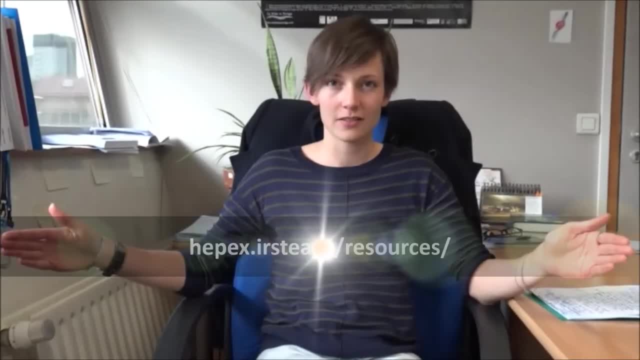 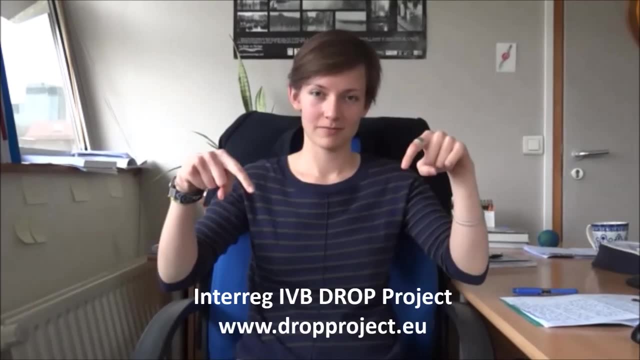 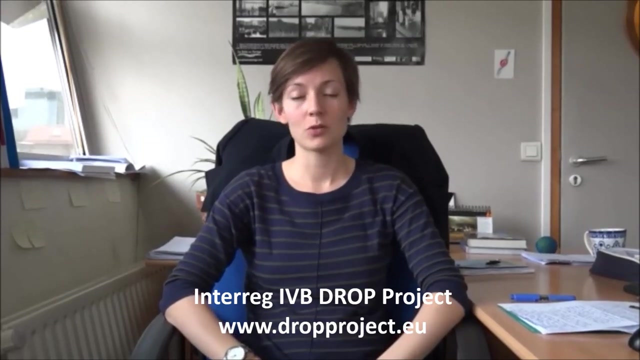 You can also find water management games at this address, If you check it out. I hope you have fun. This work is part of the Interreg for Bidrop project. The objective of this project is to help north-western European regions better prepare and adapt to droughts and water scarcity. 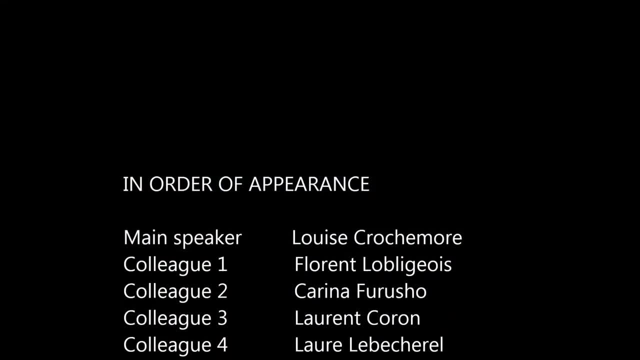 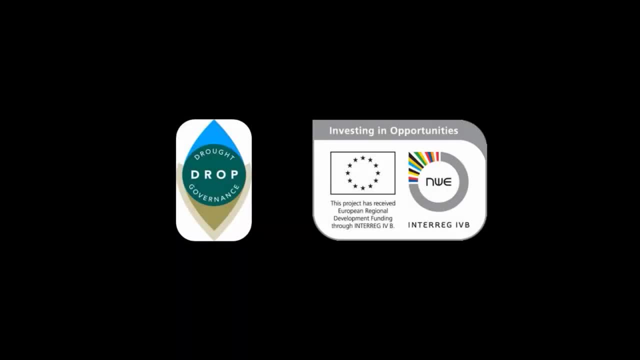 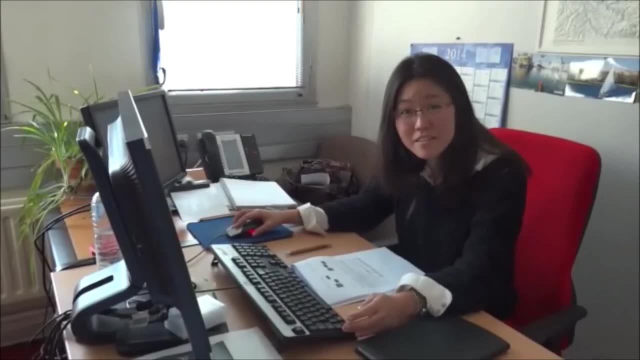 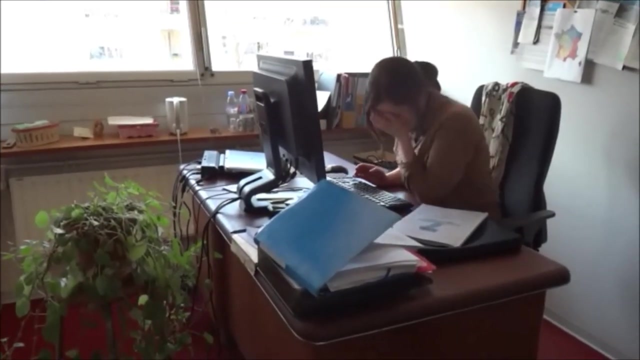 Thank you for watching Ladies Ladies Broadcast Without the pen. Is it actually working now, Uh?